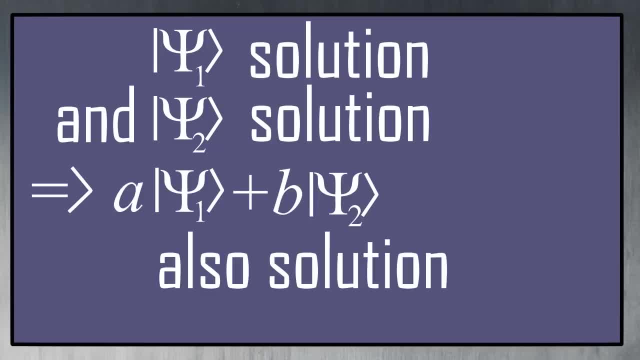 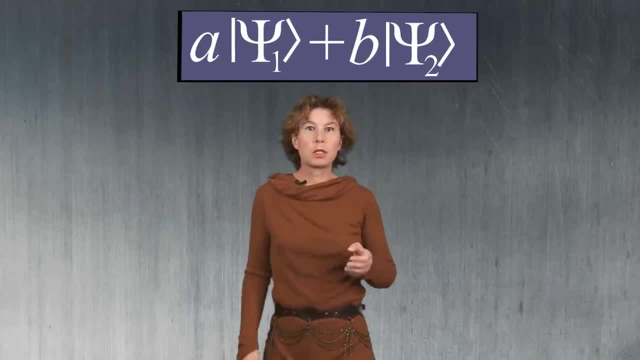 the equation, then any sum of those two solutions with arbitrary prefactors is also a solution, And that's what is called a superposition. It's a sum with arbitrary prefactors. It really sounds more mysterious than it is, But it is relevant because this means. 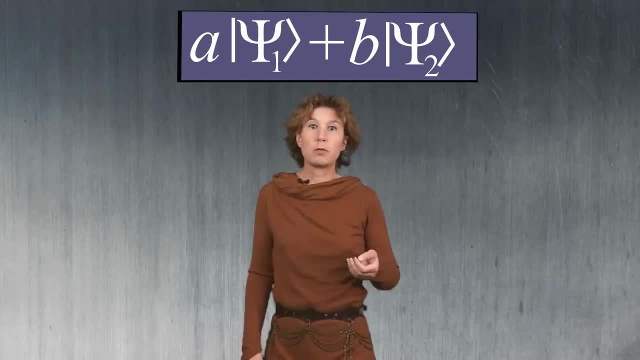 if you have two solutions of the Schrödinger equation that have a correspondence in reality, then you can also make superpositions of them, and the superpositions then should also have a correspondence in reality. This is where the idea comes from, that if the 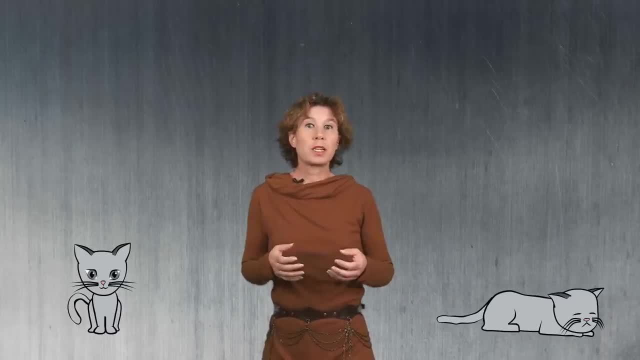 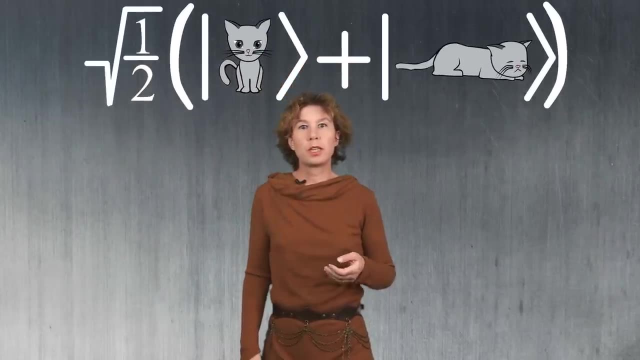 cat can be dead and the cat can be alive, then the cat can also be in a superposition of dead and alive. Some people interpret such a superposition to mean that the cat is neither dead nor alive, nor alive in reality, And that's why you want to measure it. Personally, I'm an instrumentalist. 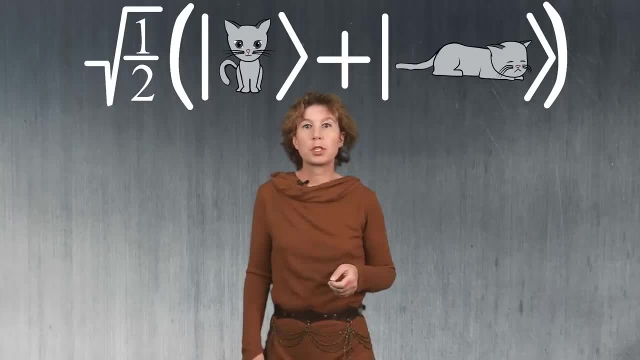 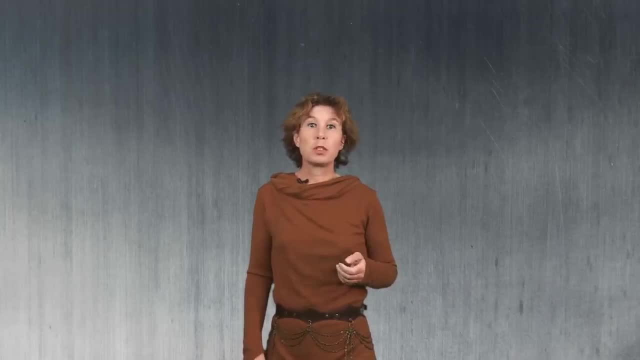 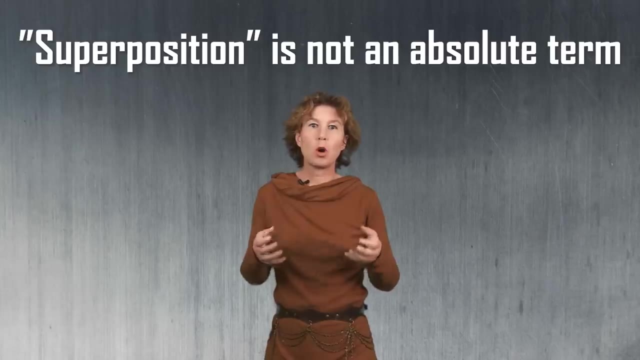 and I don't assign any particular meaning to such a superposition. It's merely a mathematical tool to make a prediction for a measurement outcome. Having said that, talking about superpositions is not particularly useful, because superposition is not an absolute term. It only makes sense to 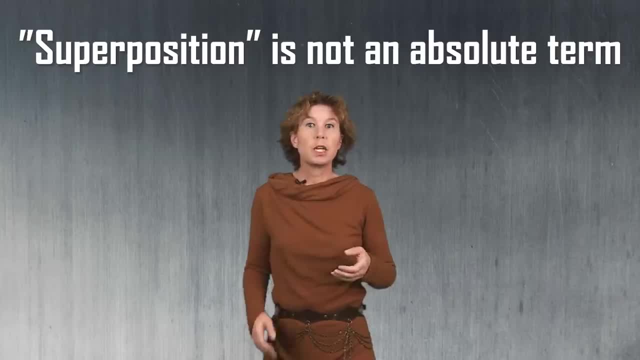 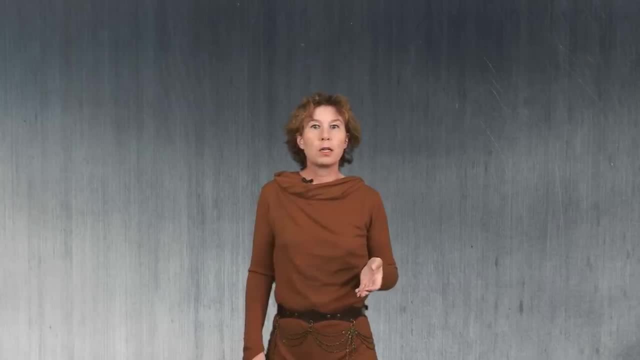 talk about superpositions of something A wavefunction can be a superposition of, But it makes no sense to say it is a superposition period. To see why, let us use the simple example of just two solutions: psi-one and psi-two. 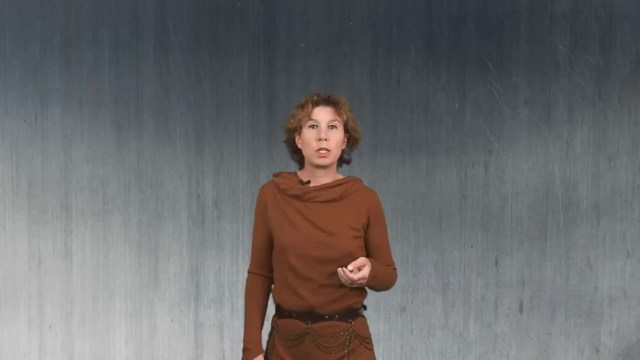 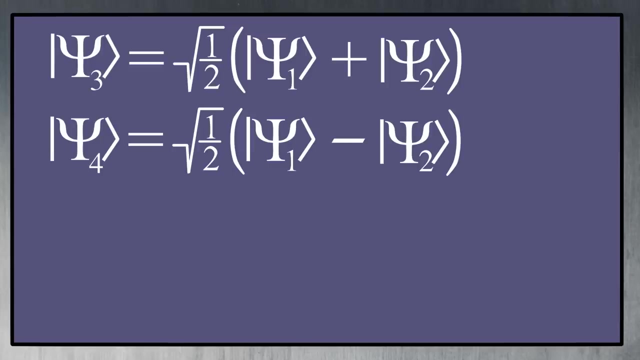 Now suppose we create two superpositions that are a sum and a difference of the two original solutions. Then you have two new solutions. let us call them psi-three and psi-four. But now you can write the original psi-one and psi-two as a superposition of psi-three. 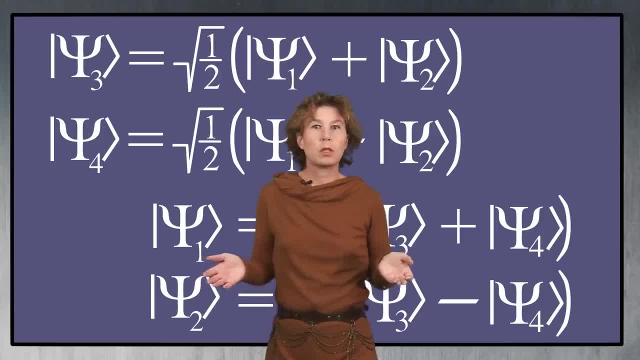 and psi-four. So which one is a superposition? Well, there is no answer to that. Superposition is just not an absolute term. It depends on your choice of a specific set of solutions. You could say, for example, that Schrödinger's cat is not in a superposition of dead and 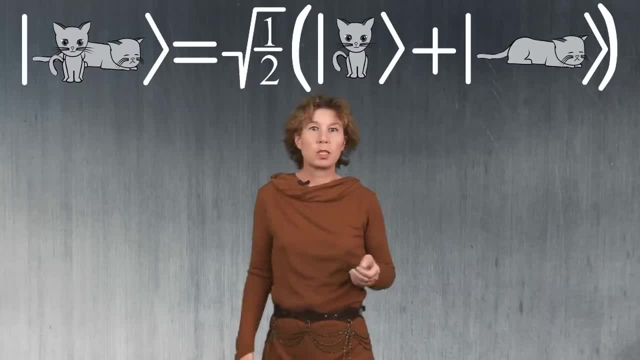 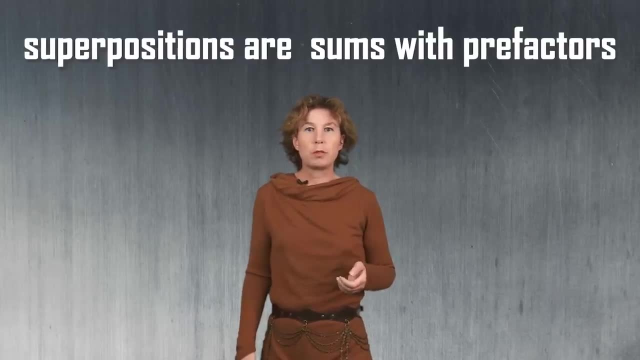 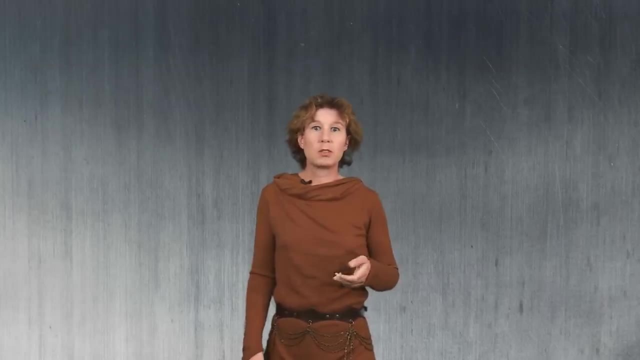 alive, but that it is instead, in the non-superposed state, dead and alive, And that's mathematically just as good. So superpositions are sums with prefactors and it only makes sense to speak about superpositions of something In some sense. I have to say superpositions are really not terribly interesting. 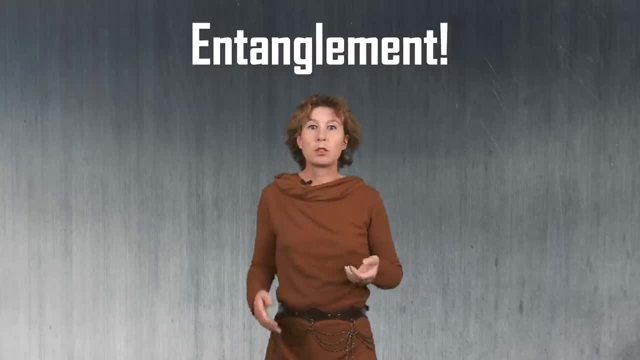 Much more interesting is entanglement, which is where the quantumness of quantum mechanics really shines. To understand entanglement, let us look at a simple example. Suppose you have a particle that decays but that has some conserved quantity. 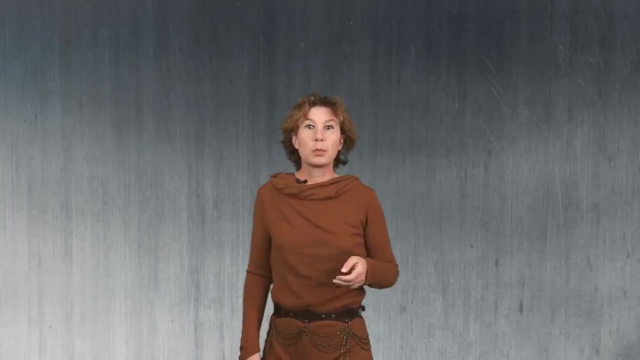 It doesn't really matter what, but let's say it's the spin. The particle has spin zero and the spin is conserved. This particle decays into two other particles. So what happens? One flies to the left and the other one to the right. 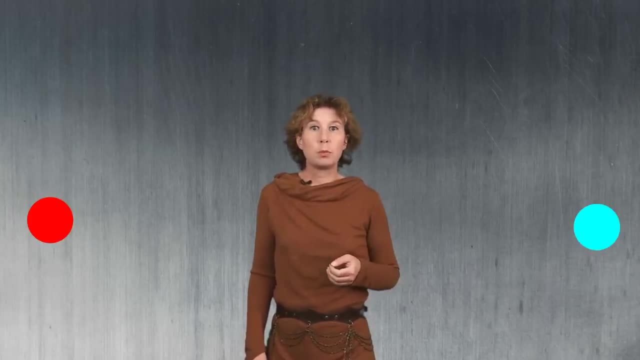 But now let us assume that each of the new particles can have only spin plus or minus one. This means that either the particle going to the left had spin plus one and the particle going to the right had spin minus one, or it's the other way around the particle. 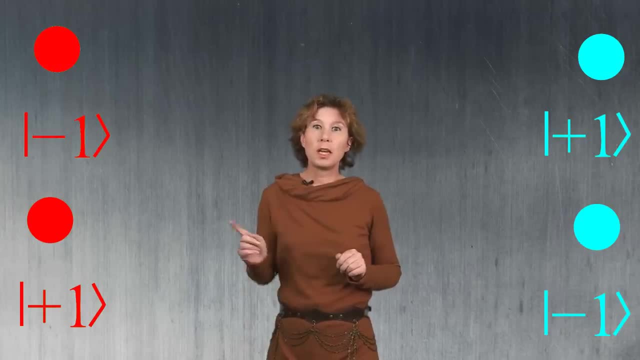 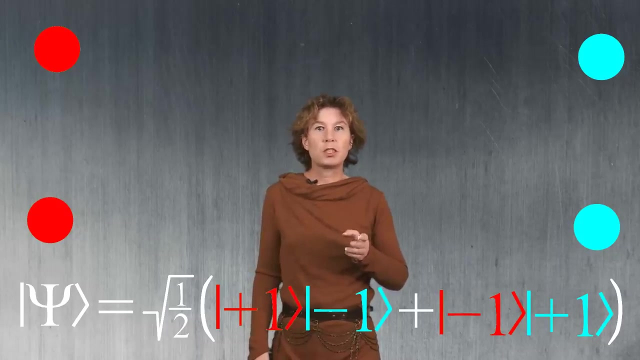 going to the right had spin plus one and the particle going to the left had spin minus one. In this case, quantum mechanics tells you that the state is in a superposition of the two possible outcomes of spin. But- and here's the relevant point now, the solutions that you take: a superposition, 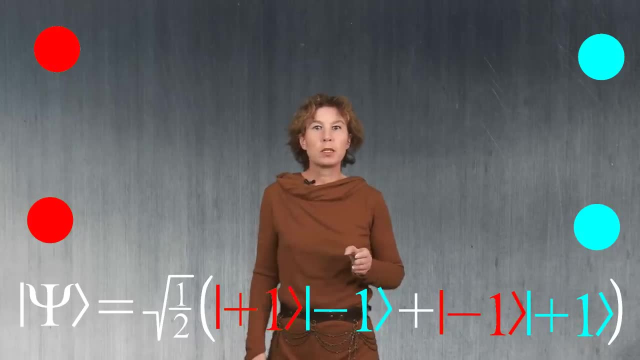 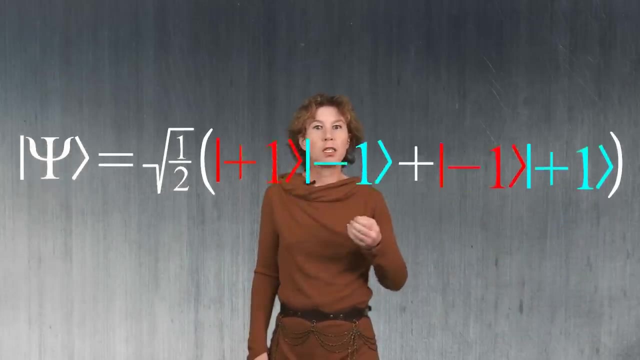 of each contain two particles. Mathematically this means you have a sum of products of wave functions, And in such a case we say that the two particles are entangled. If you measure the spin of the one particle, this tells you something about the spin of. 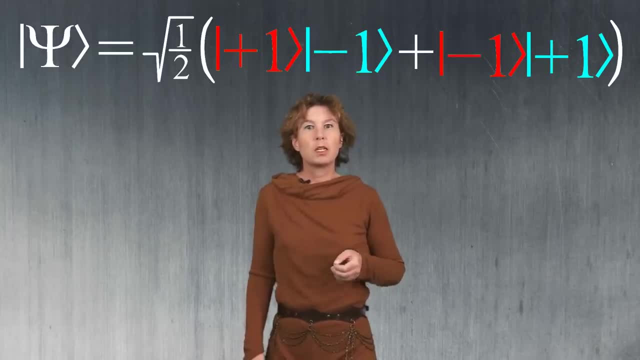 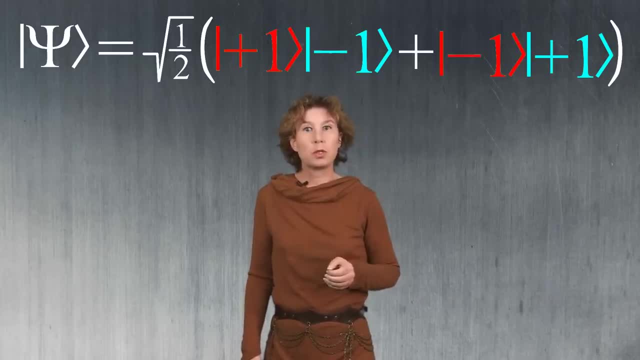 It does not depend on the way that you select solutions to the Schrödinger equation. A state is either entangled or it is not, And while entanglement is a type of superposition, not every superposition is also entangled. 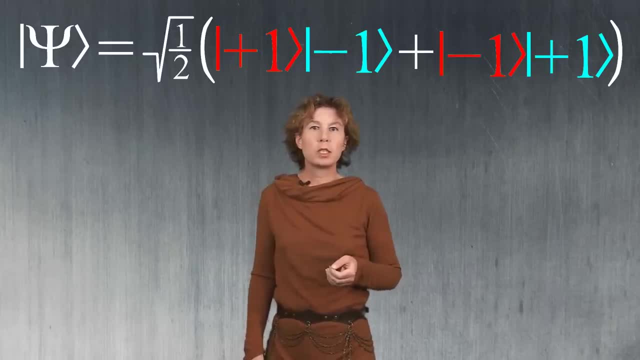 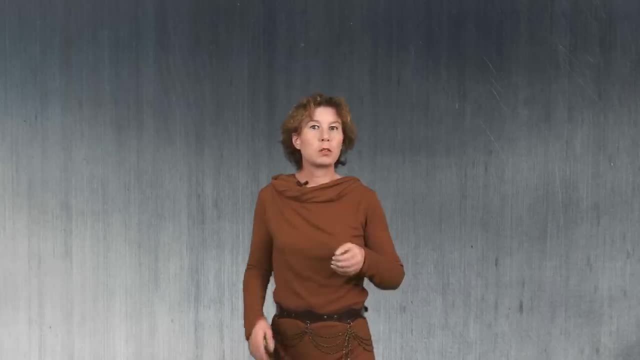 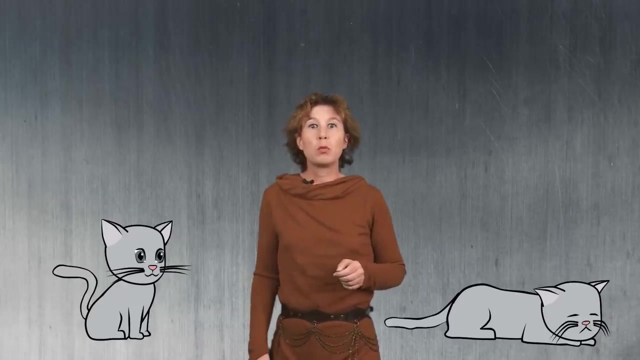 Loosely speaking, entanglement is a type of correlation that is specific to quantum mechanics. A curious property of quantum mechanics is that superpositions of macroscopic non-quantum states quickly become entangled with their environment, which makes the quantum properties disappear in a process. 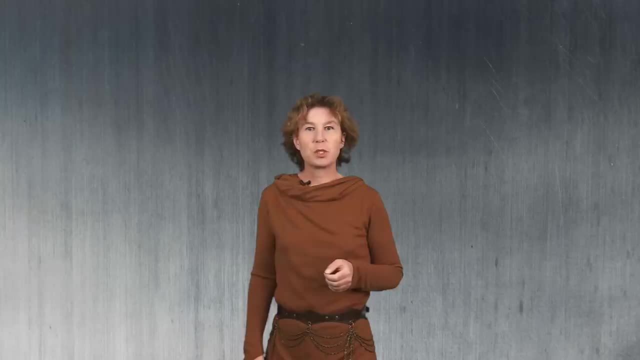 called decoherence. We will talk about this some other time, so stay tuned. Thanks for watching. see you next week. Oh, and don't forget to subscribe.